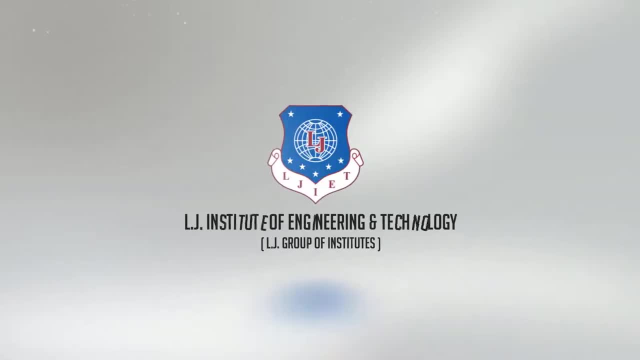 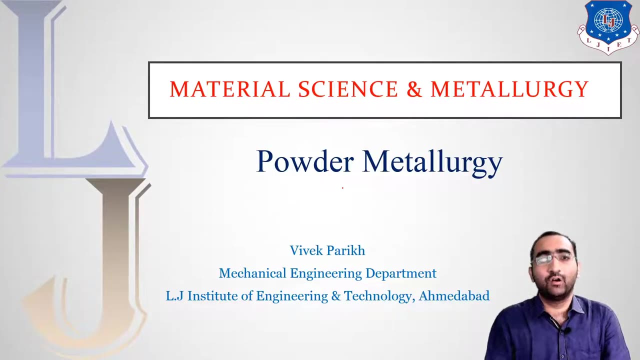 Hello students, welcome back to the online sessions of the powder metallurgy- Myself, Vivek Parikh. We were discussing the powder metallurgy in this unit, So what we have discussed in the previous lecture, we have seen the what do you mean by the powder metallurgy. We have also gone for the thing that is, the different steps which are there in the powder metallurgy, and out of that thing we have discussed the powder metallurgy. 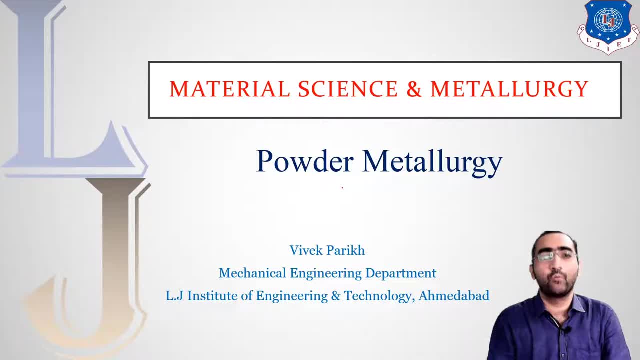 We have started our very first step. that was known as an powder production method. How the powder production methods are there. They are divided into four main categories. That was the mechanical, physical and all that things we have done. So out of that thing we have discussed all the mechanical powder production methods. So, whatever the remaining thing, that is, the chemical methods, physical methods and the electrochemical methods that we will be discussing in our today's lecture. So let us begin this lecture with the thing that is the powder production method. 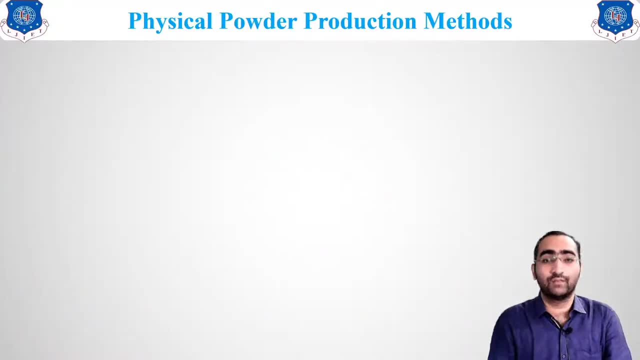 That is the powder production steps, and out of that powder production, the second method which we will be starting, that is known as a physical powder production method. So what is this physical powder production method? This method is the thing due to the physical changes That means we are changing almost the state of the matter we are changing. and out of that thing, the very first method we will be seeing that is known as a condensation method. What do you mean by the condensation? as the name suggests, 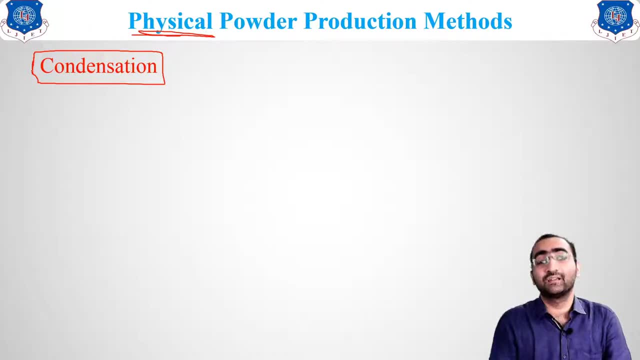 Condensation means we are converting the particular gases into the liquid and from that liquid we will be condensing to the solid. So this method, or this aim, we will be taking and we will be going for the powder production. So the first method which we will be using, that is known as a condensation method. You are aware about the thing condensation. Okay, So the same thing. we are applying it over here. So what is the thing? This method employs? to the principle of condensing the metal vapor to obtain the metal powder. 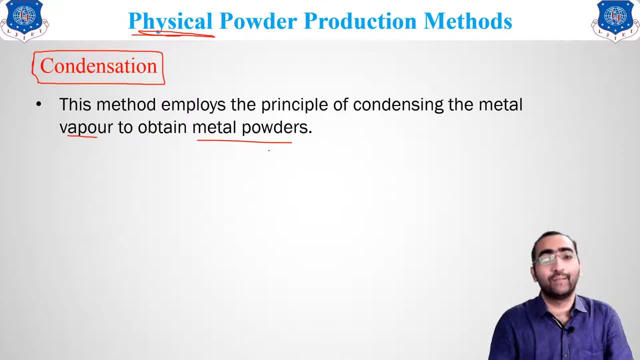 As I told you, the vapor will be converted to the metal powder. Now it is what this method is suitable for: the volatile metal which are transformed into vapor easily. That means metals are very difficult to get converted into vapor. So this method is not employed to each and every metal. It is only done on the certain metals. Why? Because each and every metals boiling point is so much higher, So it is not an economical thing and we require such type of the furnaces to convert it into that particular metal. 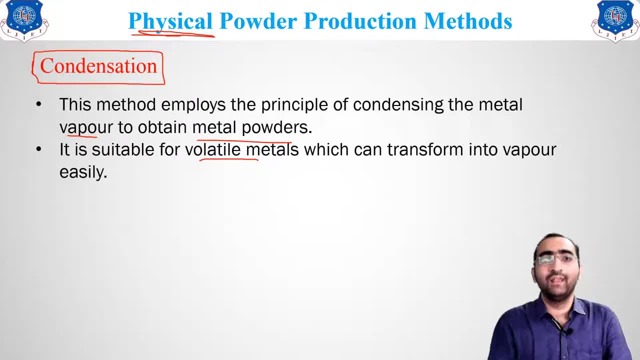 Part, So it can be employed whose boiling point is less for that material only we can use this condensation method. It is carried out in the controlled atmosphere to avoid the formation of the oxide, So that what we are doing, we are going for the condensed. That means the controlled atmosphere. we will be going Why? Because if there is not a controlled atmosphere, what will happen? Your metal will react with the oxygen of the atmosphere and, as a result of which, what will happen? the oxides will be formed. So to avoid that oxides, we will be going for the condensed. 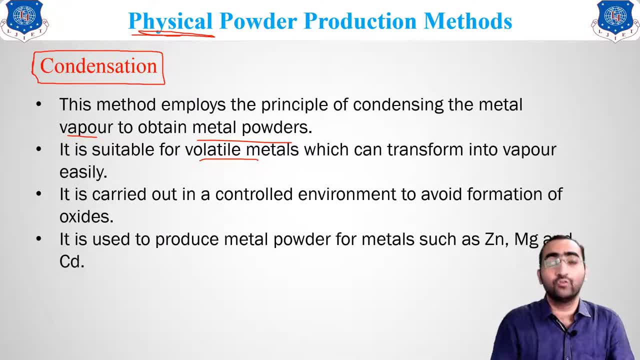 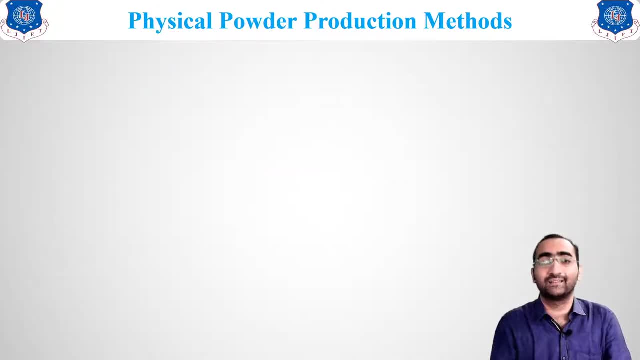 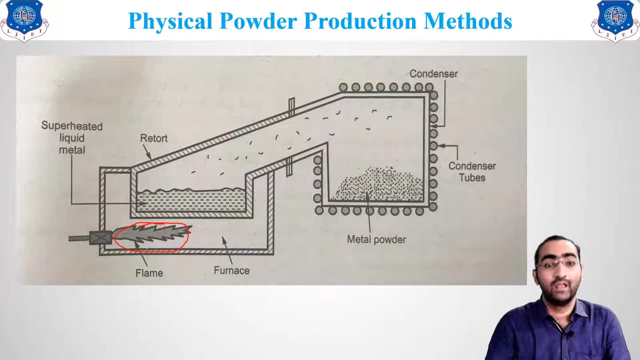 For the controlled environment for which metals we can use. we can go for the powder production method for the zinc, magnesium, cadmium. Why? Because their boiling points are less clear. So now let us see the figure. How does it happen? So this is the figure. here There is a flame generation, is there? This flame is generated? What will happen? due to this thing, This metal pieces will convert into this liquid form and out of that liquid it will start into formation of the gases. These gases will move. 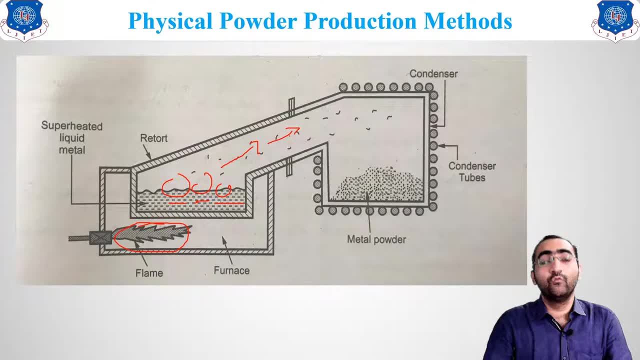 What Gases has a tendency that it will move away wherever the space is there. So it will move in this way over here and here you can see condensers are placed. So what will happen? There is a temperature drop will be there, So this vapor will fall down as a part of a liquid droplet and during the falling and during this cooling, what will happen? It will convert into the powder and you can see the metal powder will be there at the bottom. So this is how you can create powder. 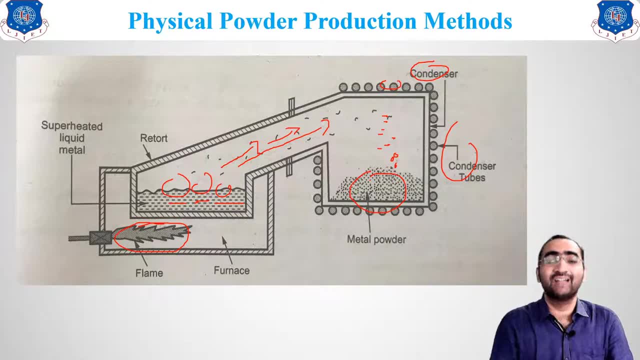 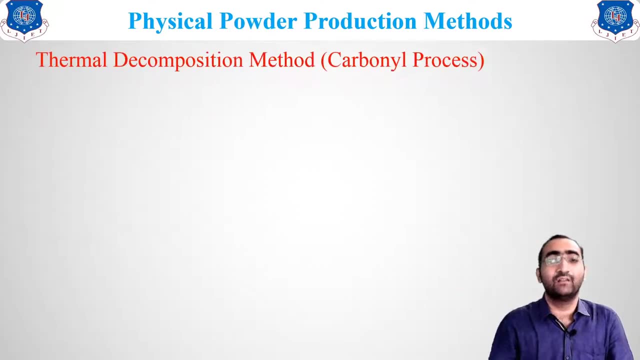 From the metal with the help of the condensation method. Clear. So very first method of the physical powder production method. Now comes the second one, that is, the thermal decomposition. Its second name, that is carbonyl process, The second one. Now, what do you mean by the carbonyl? You might be aware about the thing: oxides, hydride. That means the metal reacts with the oxygen. It will give you oxide metal. reacting with the hydrogen gives you hydride halide. 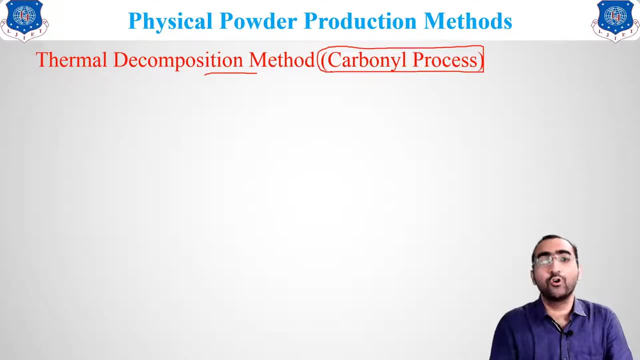 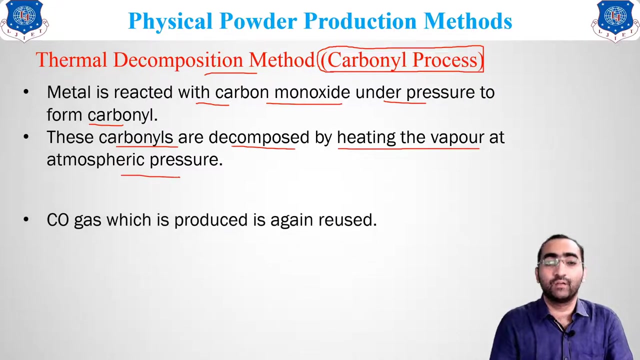 The same way, when metal reacts with carbon monoxide, the material which is formed that is known as an carbonyl method. So we will be using that technique. in this method, Metal is reacted with carbon monoxide under the pressure to form the carbonyl method. Clear, As I told you. Now, this carbonyl, they are decomposed by heating the vapor at an atmospheric pressure. The CO gas which is produced is again reused. So let us see, this is the equation. 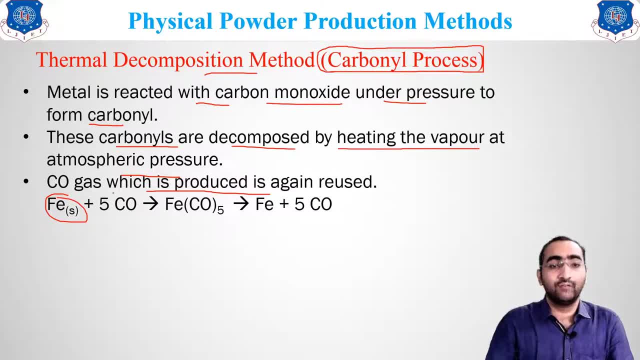 solid, it is a bulk. we are reacting it with a fico, that is, carbon monoxide. so what will happen? we will get a carbonyl. carbonyl has a tendency. they are brittle in nature. so when you get iron carbonyl, heat the material with the hammer and all what will happen? it will disintegrate, it will. 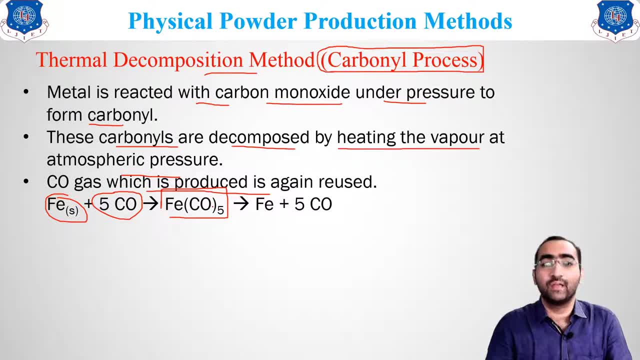 disintegrate and a small powder particles will be get after that. which particles you are getting? the particles which we are getting, they are of the iron carbonyl, so we have to remove the carbon dioxide. so what you will be doing, go for the heating at a high temperature. what will happen? 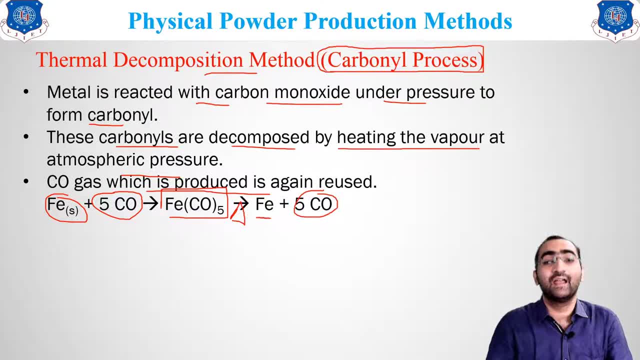 your carbon monoxide will go away and we get the iron. this is a bulk iron, this is a powder iron we are getting and this carbon monoxide is once again reused for the next batch. so this is how thermal decomposition method works. which are the thing metal, majorly iron and nickel. they are the metal which can be, probably can be produced with the 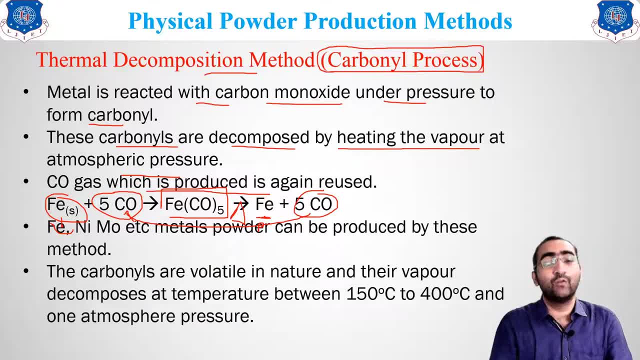 help of this, carbonyl processes clear. the carbonyls are volatile in nature and if the temperature range which takes place, that is, between 150 to 400 degrees Celsius and one atmospheric pressure, that means we can achieve this method very easily as compared with the condensation method. so this 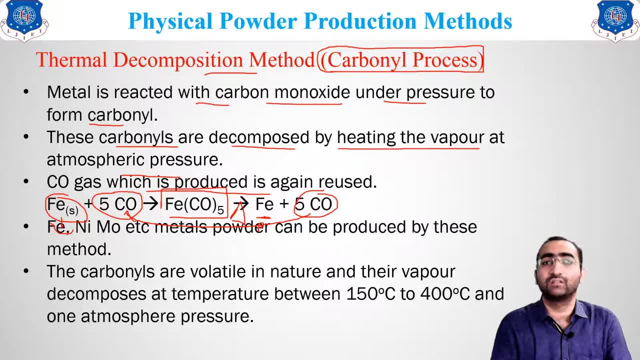 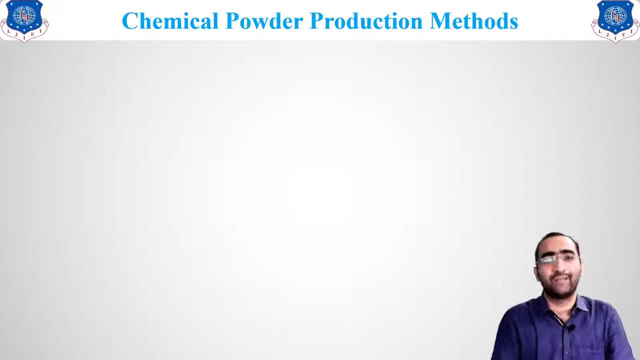 was our second method of the physical powder production, that was, the thermal decomposition decomposition method, and there are only two methods which are there for the physical powder production method. Now we will be going with our third category of powder production, that is known as a chemical powder production method, and in that let us start our very first thing, that is, 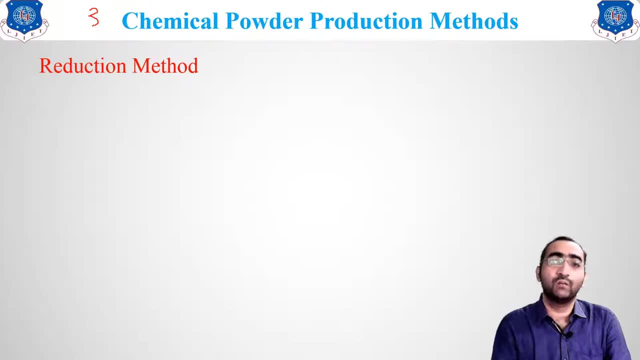 the reduction method. You will be aware about the term reduction. What do you mean by the term reduction? Reduction is nothing but removal of the oxygen or adding of the hydrogen. that process is known as an reduction method. So if you are adding hydrogen, what will happen by addition of? 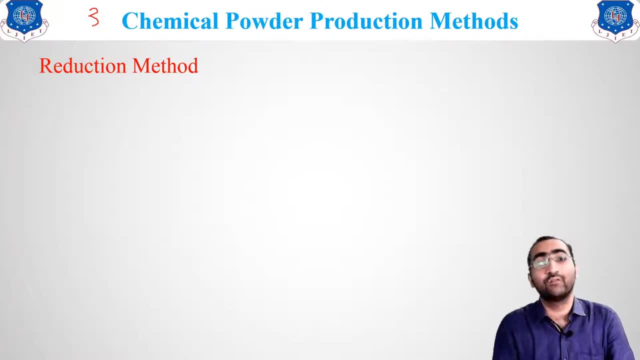 the hydrogen, you will get the hydride. Hydrides has always a tendency of a brittle in nature. So we will heat the material, disintegrate the material and we will get the thing that is the powder of the material. So this method is based on the principle of breaking. 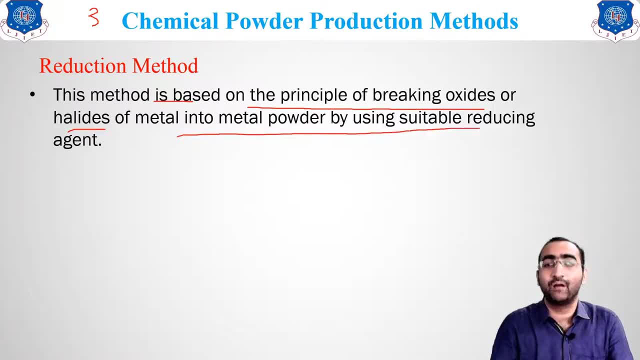 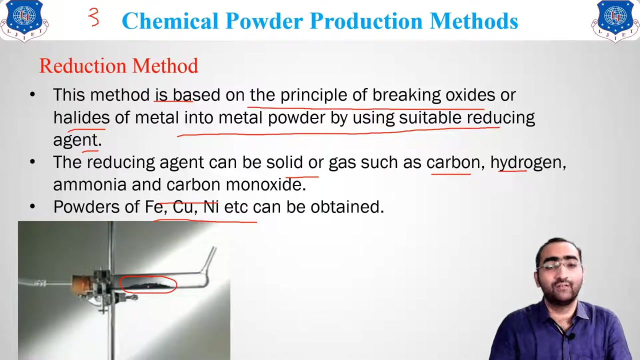 oxygen. Now the reduction agent can be solid or a gas, as carbon hydrogen, ammonia and carbon monoxide. So powder of iron, copper, nickel. they can be obtained with this reduction method. So you can see over here copper we are taking. Copper has been reacted with a carbon monoxide or you can. 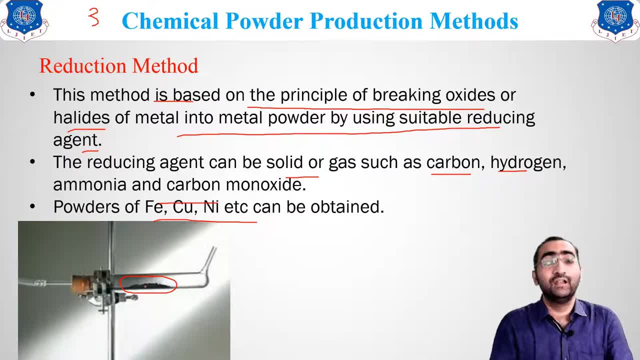 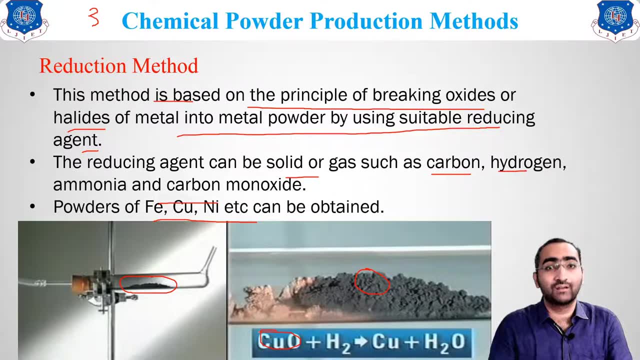 say coke, and after that what we will be seeing by the introduction of the reduction method is that hydrogen. you can see this particular thing. see, this is the thing. CuO, copper oxide metal- is there. then with the help of the hydrogen, it will reduce. Here there is a pure copper, so you can see copper. 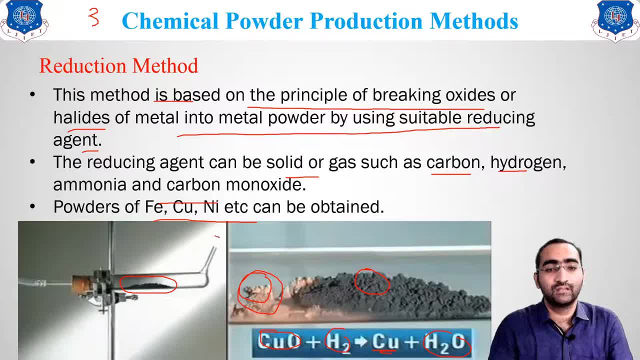 plus H2O gas. this gas will goes away from here and whatever the thing which is left, that is your pure copper. take this copper, heat the material and you can go for the particular powder from this material Clear. So that was everything. so thanks for watching. See you next time. bye. 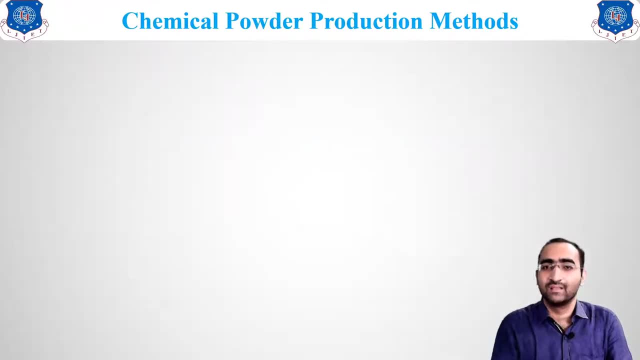 If you are using short of a bomb, Do not smoke before she's. You can have the stuff from within clear. so that was the reduction method. second method which is there in the chemical powder production, that is the intergranular corrosion. intergranular corrosion- what will happen? we are 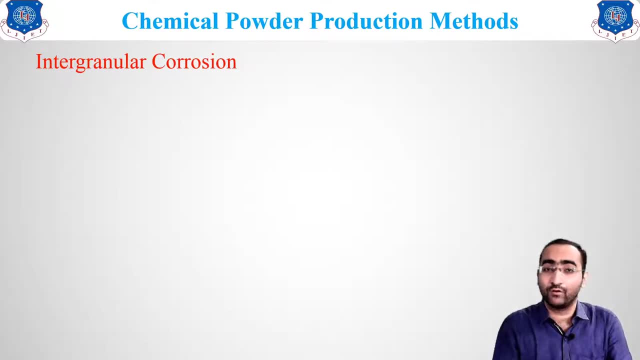 intentionally going for the corrosion. how we are going for the corrosion, that is, the between the intergranular grains, between the two grains. we are going for the corrosion. so what will happen? your material will become brittle and as a brittle heat, the material you will get, the powder- the same. 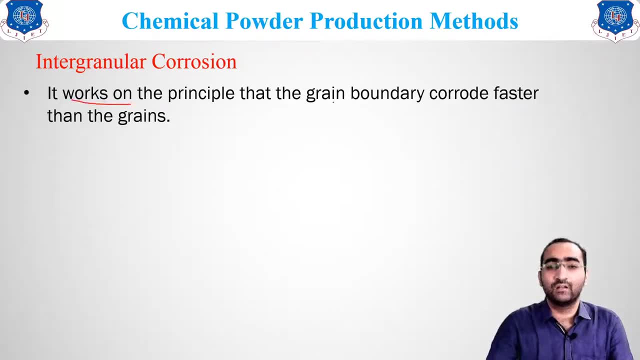 things applies over here. you can see it works on the principle grain boundaries corrode faster than the grains as, comparing the grain boundaries with the grain, your grain boundary will get corroded faster. so the grain boundary, area of metal corroded by suitable electrolyte. so what we will? 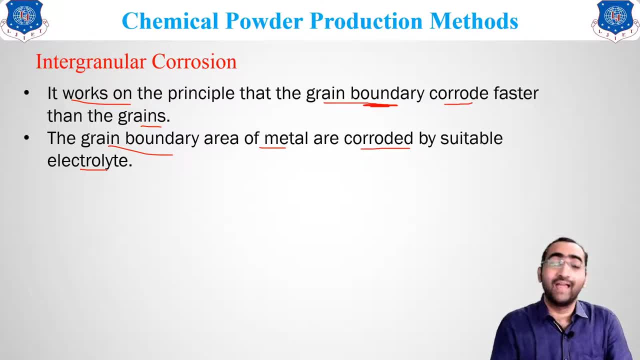 be doing? we will be taking some electrolyte and, as a result of that electrolyte, what will happen? that electrolyte will give the corrosion in the grains between the grains. due to the corrosion, the grains separates out in the form of polycrystal and metal. due to that, 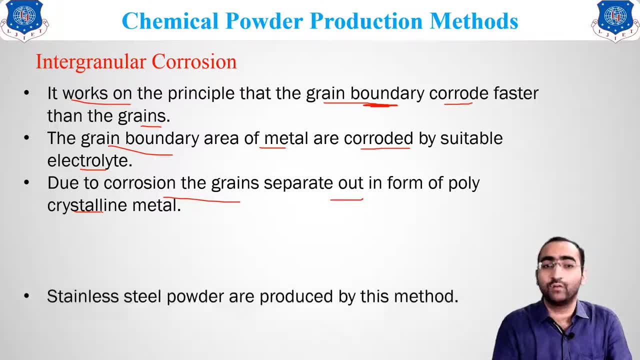 what will happen? the grains goes away and there is a gap between the two grains. stainless steel powders are produced by this method. so due to that thing, what doing? by the corrosion, we are taking away the grains, we are taking the between grain boundaries and due to that, there is a space. 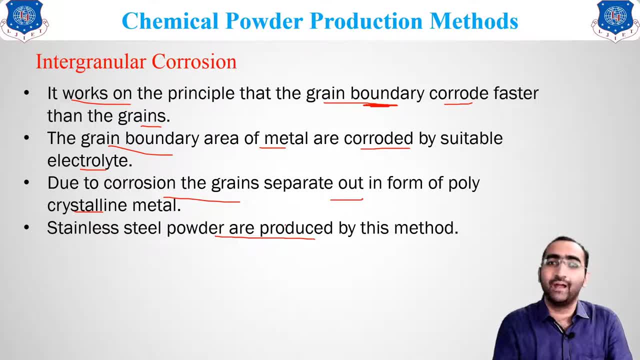 which is there. so the material will become a brittle and by heating it, what you will get? we will get a metal powder from this thing. you can see over here we are doing this thing, so cracks will be formed. why this thing happens? these are the different grains which we have corroded, so 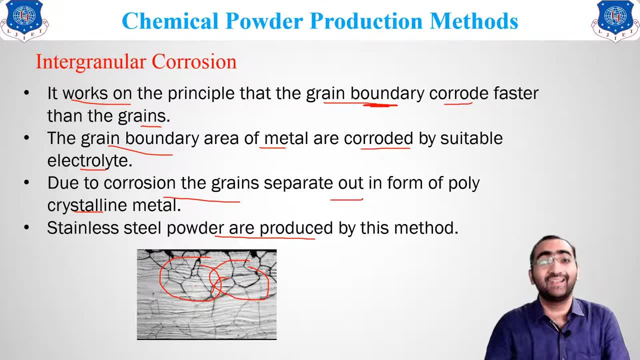 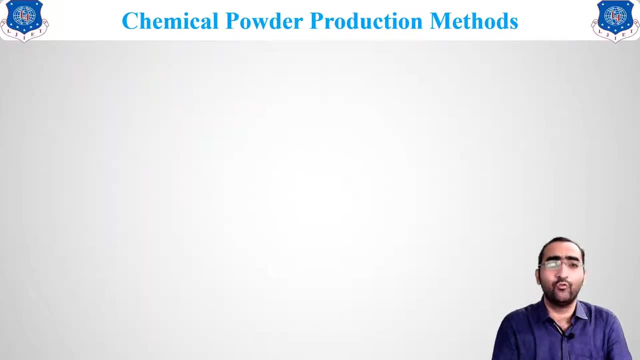 what has happened? the material is having a cracks. due to that crack, it is easy to get break down. so with the help of this method, we can go for the powder production- major stainless steel materials powder. they are manufactured with the help of this method. clear, now going for the third method. 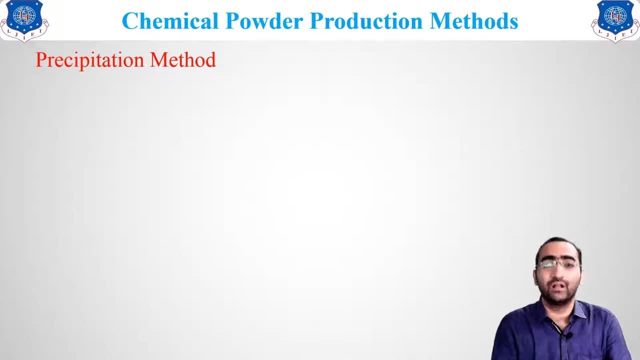 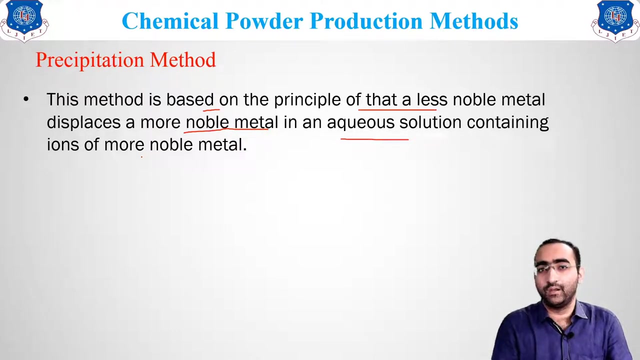 last method, third last, that means the last method of this chemical powder production, that is, the precipitation method. this method is based on the principle that a less noble metal displaces the more noble metal in an aqueous solution. now you will be knowing about the precipitate that the material will get. 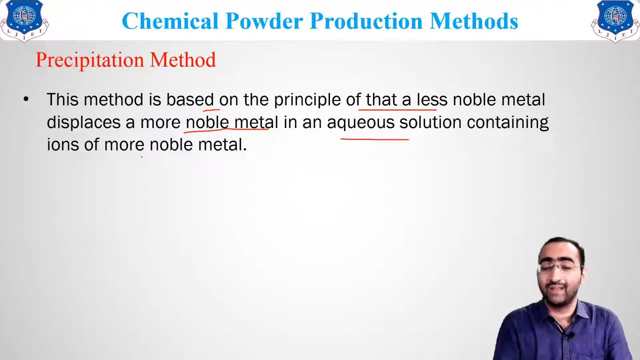 bulk with each other and the precipitates are formed, and that precipitates. by using that precipitate, we will be going for the powder production, the more noble metal the separates out in the form of a powder production, and that is how we are going to get the precipitates. 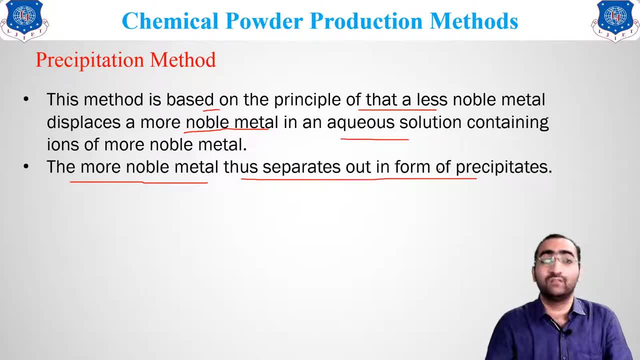 form of precipitate. that means whatever the material we are having which will behave as a more noble metal, that will get the precipitates and it will settle down at the bottom. So AG, SN, CU, these are the metals which we can use, this thing and the precipitate, whatever we are getting. 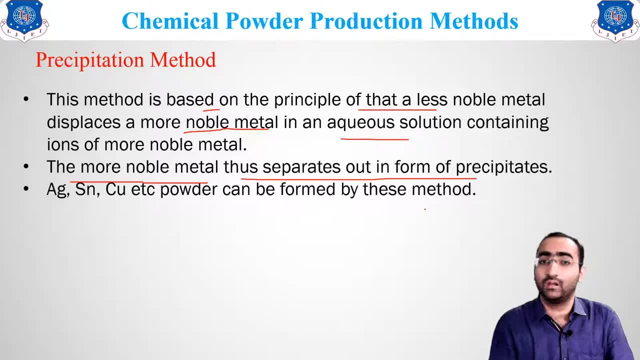 they are always brittle in nature. take that, precipitate, heat the material. you will get the powder from that particular thing. So this was your precipitation in all the three things: intergranular corrosion, what we did, we did, a chemical reaction. in this precipitation, what we are doing, less noble and more noble metal are separated out with the help of the electrolyte and 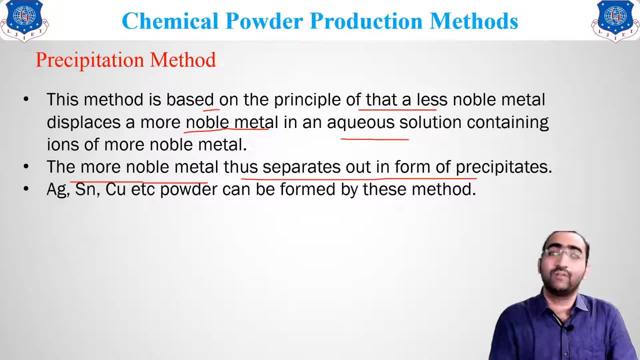 all and due to that chemical thing, we have done what we have done. we are going for that thing and the third method which we have done, that is the reduction. it is also one of the chemical reactions which is taking place that mean there are three methods in the chemical powder production. 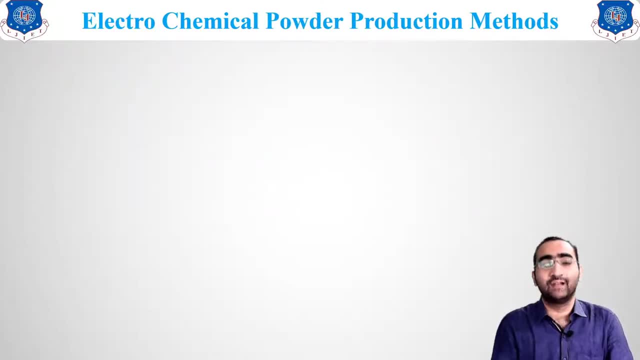 method. okay, and the last method, that is, the electrochemical powder production method. how does it happen? it uses the principle of the electro deposition and electroplating. you will be knowing that: a silver on a copper spoon if you are going for the silver, silver plating and 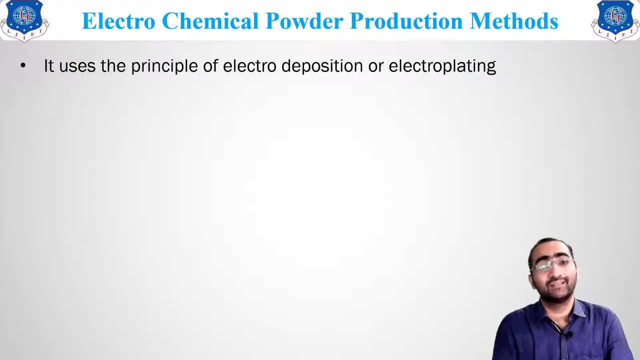 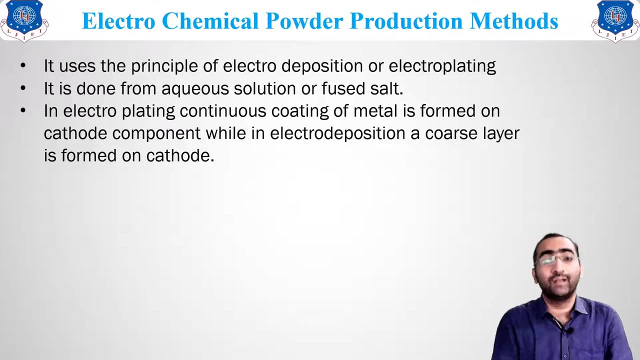 all that is done with the help of the electro deposition or electroplating, the same method. we are applying it over here. it is done in the aqueous solution, how we are doing. we are going for the plating. continual powder can be obtained in the three ways: either the first one, that is, 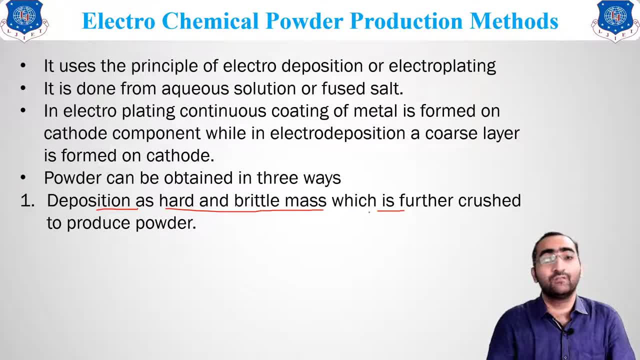 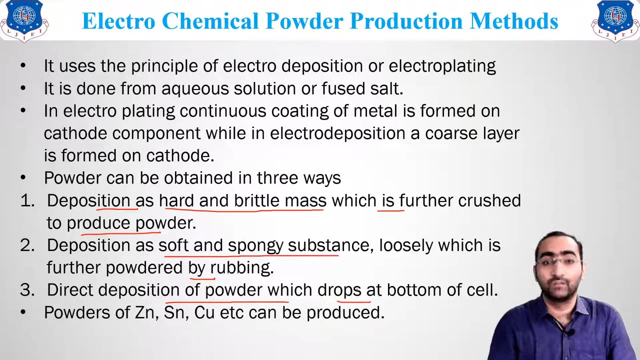 the deposition as hard and brittle mass and which will be further crushed to the powder. second one: deposition as soft and spongy substance. with the help of rubbing we can remove it. and the third one, that is, direct deposition of powder drops at the bottom. let us see how it happens. which metals are prone for this thing. that is the. 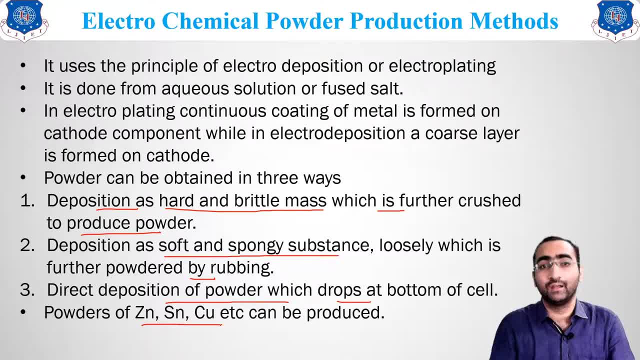 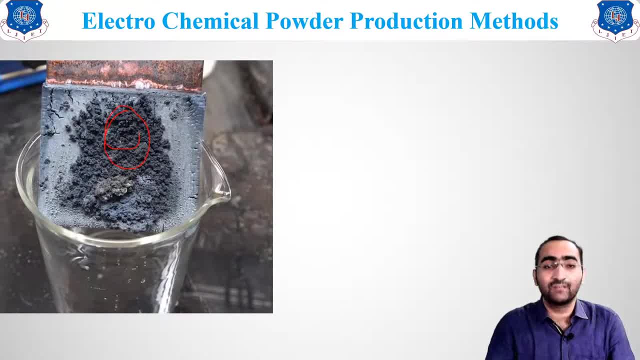 zinc, tin, copper. that type of the material, the powder, can be found with the help of this method. let us discuss it with the help of the figure. here you can see: soft and spongy. this is the second one. first one, hard and brittle metal which is there on the material, and the third one that 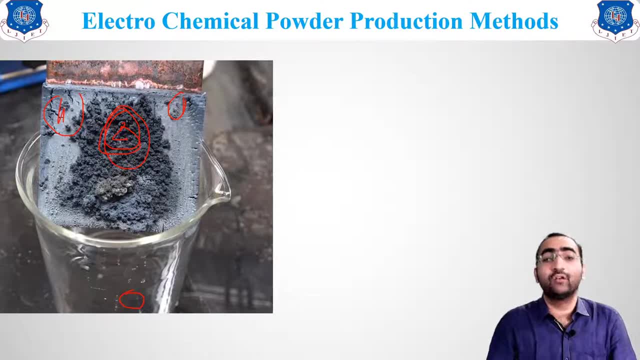 is obtained at the bottom which are not able to get on this particular surface, and this is your anode and this will be your cathode. so what you are seeing, you are seeing that anode was used and the cathode, that is the zinc material, is based on this material and by rubbing this thing, what you 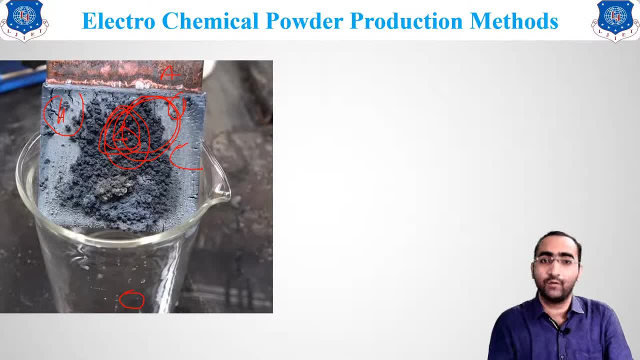 will get, you will get the powder. and whether you are not getting the powder, it is a brittle in nature, so you will get the powder. so by removing this metal, what you will get, you will get this particular metal as the soft and the brittle material hit the material, get the powder and the powder will be with you. clear. so this was. 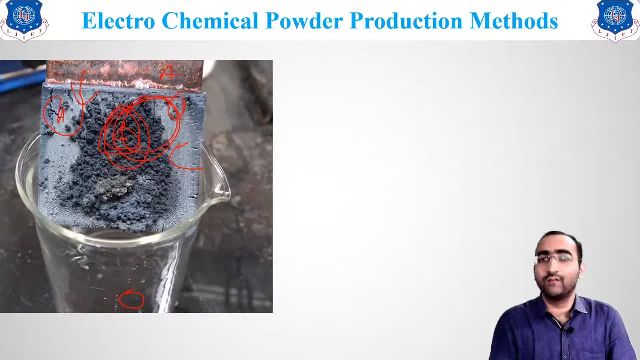 your electrochemical method and, as a result, what we have done. we have done or we have discussed all the powder production method. they are physical, chemical and electrochemical in this lecture and we have already discussed the mechanical one. that is, in our previous lecture, clear, So now let us discuss it with the help of the second going. this is the basic set of anode cathode. 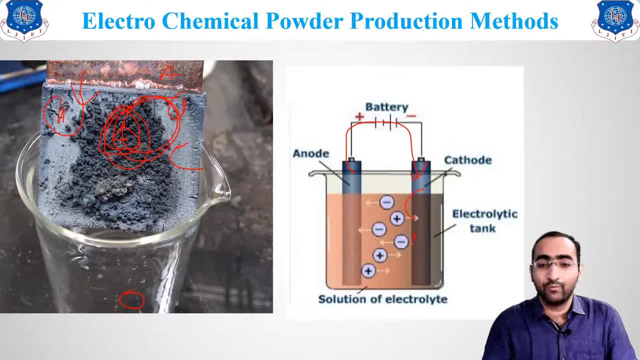 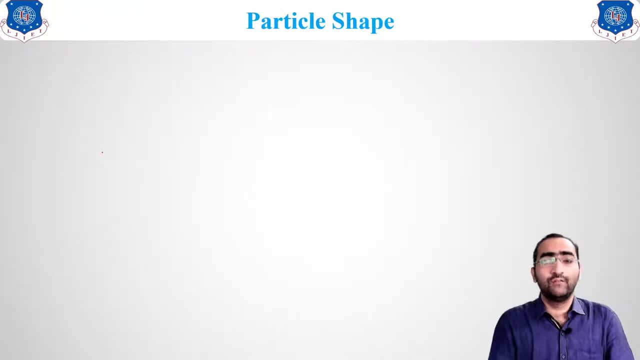 this anode will be depositing on the cathode and will deposit in this way on this particular material. in this way we can find out this thing. So we will be going that. which are the different types of the particle shape we are getting? which type of the shape? spherical, rounded, cylindrical, spongy, aggregated, cubic, flaky, acicular, how it look like. 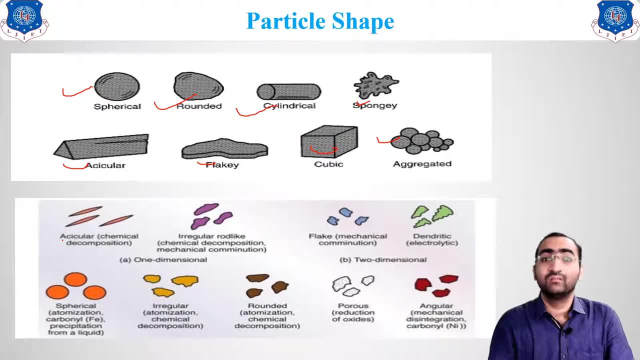 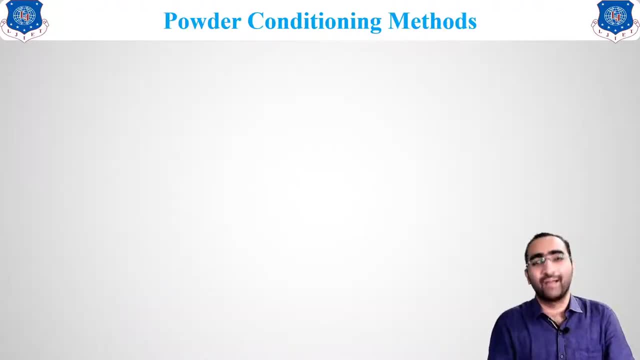 They are, in this way, three dimensional view. you can see, this is how you can get the different types of the particles which are getting from the particular powder production method clear. And now we will be starting with our second step of powder metallurgy, that is known as. 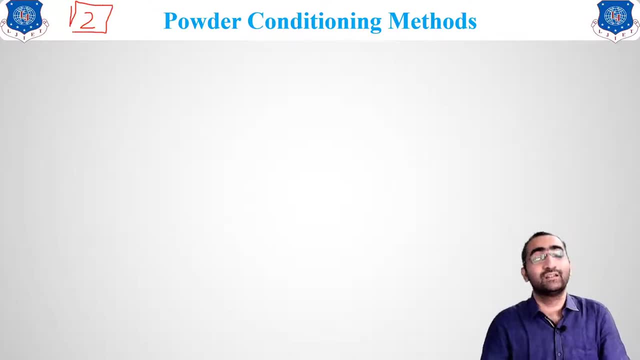 an powder conditioning method, as we have discussed in the last lecture. what is this powder conditioning? that is nothing but mixing of the different types of the thing. why let us see powder conditioning, That is, of the two types, either mixing or blending. these two things we can do. what is blending? 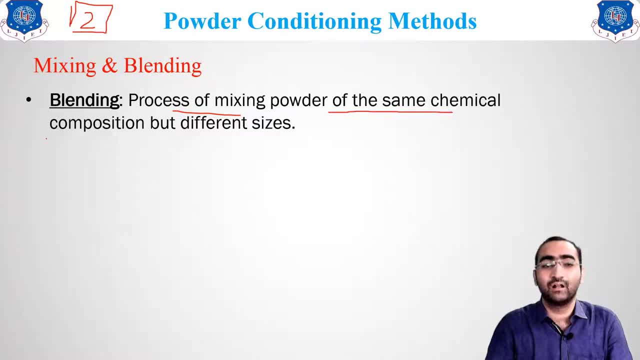 process of mixing powder of same chemical composition but different size, same chemical but having a different size, whereas mixing means process of combining two different powder chemistry. if we are taking the two different things, that means alloy if we are using, we will be going for mixing. if it is a pure metal, we will be going for the blend. 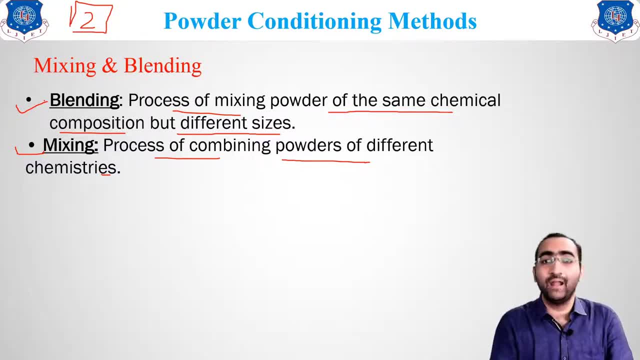 But clear basic difference between mixing and blending. mixing take two different metal, blending the same metal, but different sizes. three things we are adding. why we are doing this thing? for the three things, which are the three things? they are the additives, binders, lubricants. binders will help us for the binding of the particles. that means it will get closer. 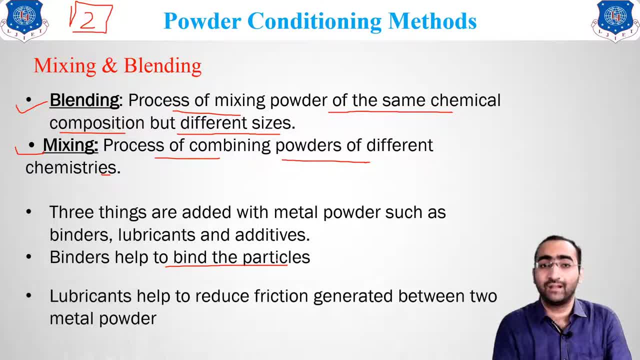 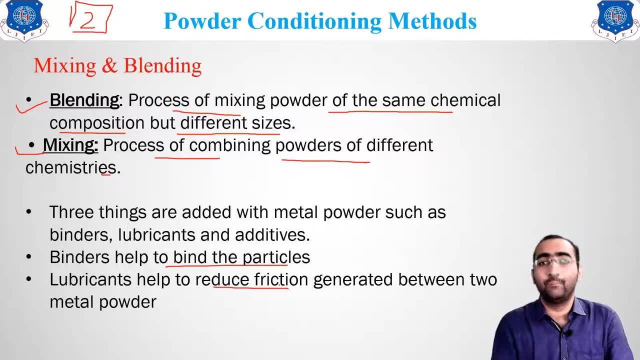 particles and will stick the particles with each other. The metal particles Lubricants. they are used for the reducing friction we are using metal. whenever the metal powder will get nearer to each other and they will rub with each other, the surface will getting rub with each other. what will happen? the friction will be generated. to avoid that friction, we 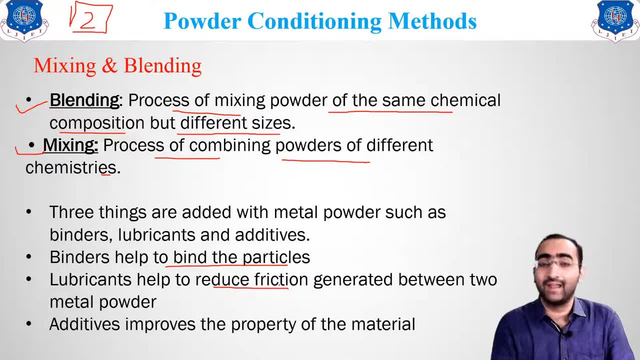 are using lubricant. the third one, additives. why? additives for the improvement of the properties of the material. so three things: we are adding lubricant for joining or sticking purpose. second- sorry, binder for sticking purpose. second one, lubricant for the friction, less thing. and the third one, additives to improve the properties of the material. 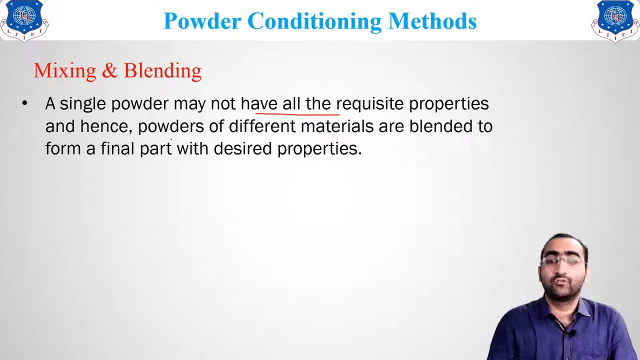 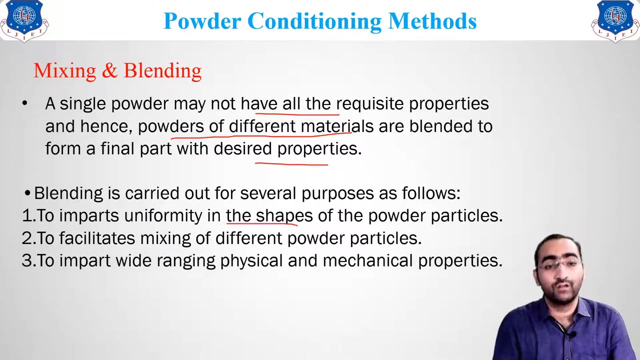 Now, a single powder may not have all properties. so what we are doing? the powder of different material are blended with each other for the desired properties. so why the blending? to impart uniformity in the shape of the powder particle, to facilitate the mixing of different powder. 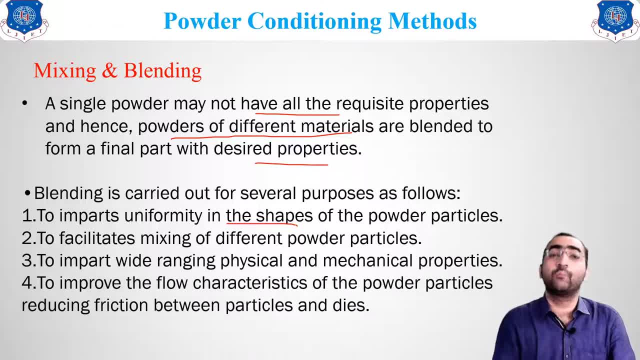 To impart the wide ranging physical and chemical properties to improve flow characteristics of the material. so these are the things why we are carrying out the mixing and blending thing. and the last one, to increase the green strength, that means the strength, by adding the binder. then on, what will happen? they can resist their shape certain and they will not. 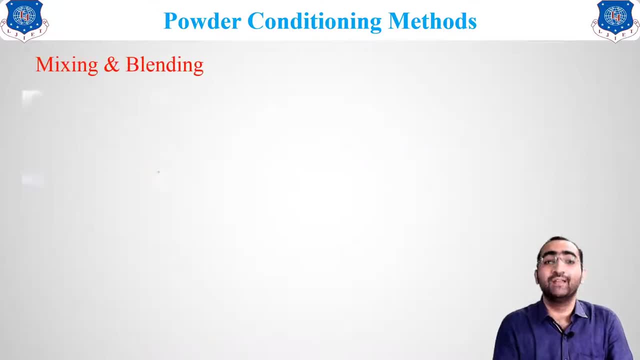 get break down how we can go for the mixing and blending the different types of the things which are used. that is the rotary drum in this drum. this drum is allowed to move. so what will happen? all the things will get mixed with each other. then there is a rotating cone rotating. 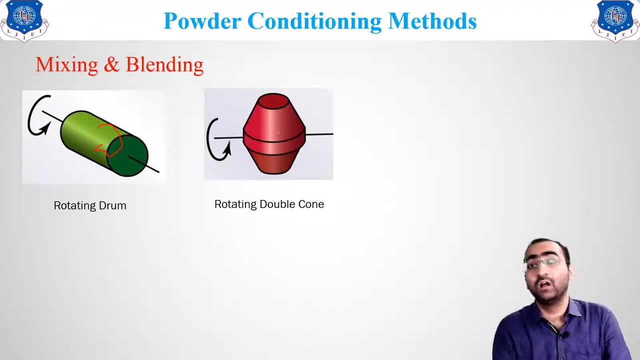 double cone here, rotating double cone you might have seen in the cement mixer machine. that is this type of the things. so it will move and, as a result, the mixing will take place. then there is a particular blade. type of the mixture is there, so this blade is allowed.